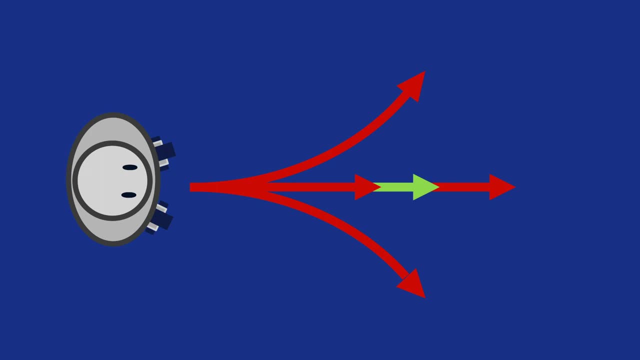 This can be because the floor is slippery, or maybe the wheels don't drive at the same speed. In other words, the robot might end up in the right place, or it could end up here or here or here or any of these places. 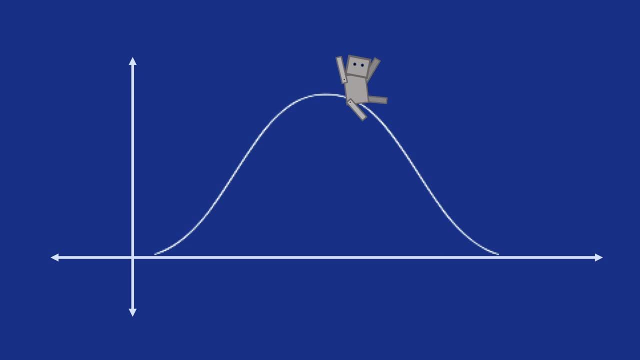 This graph can tell you how to make your robot do things totally wrong. In this case, the location of the robot is along the bottom and the likelihood that the robot is at that location is on the side. This curve is called a Gaussian curve after a guy named Gauss. 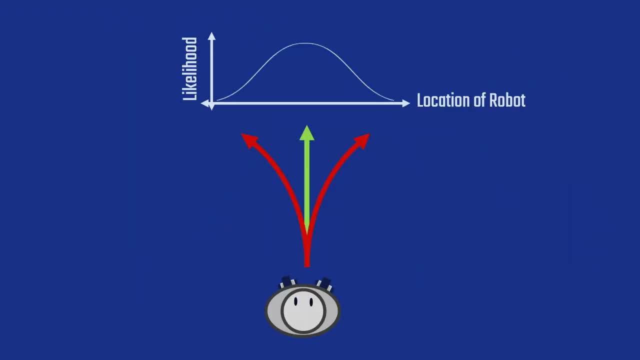 But it's also called a bell curve. When the robot moves, it's most likely to end up where it's supposed to be, but it's also very likely to end up near where it's supposed to be. It's unlikely to end up far from where it's supposed to be, but it could be there In. 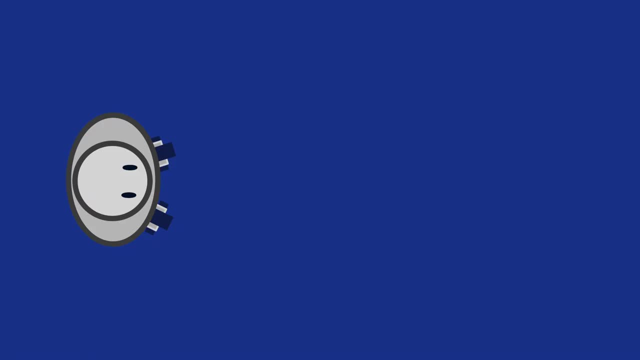 fact, the robot could wind up anywhere. The robot's sensors are also really terrible. The sensors tell you how far away the next wall is. If that wall is, say, 30 inches away, the sensors will tell you that the wall is 29 inches away, or sometimes. 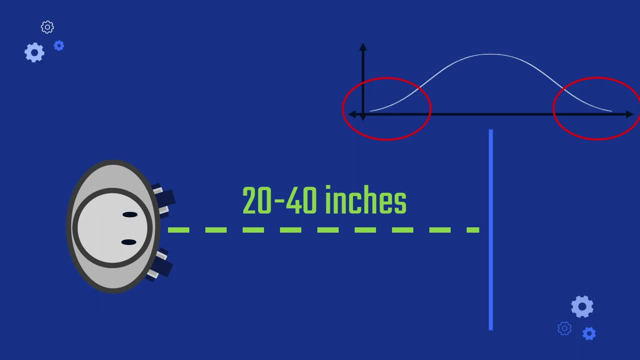 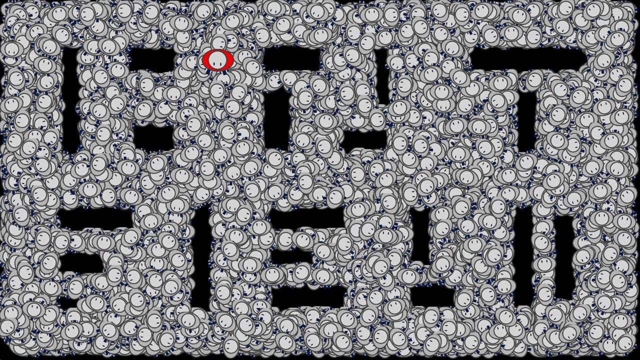 it'll tell you that the wall is 20 inches away In the simulations. each of these robots actually has nine different sensors and all of them are terrible. So you can now move lots of robots really badly and you can read lots of sensors really badly. How does this? 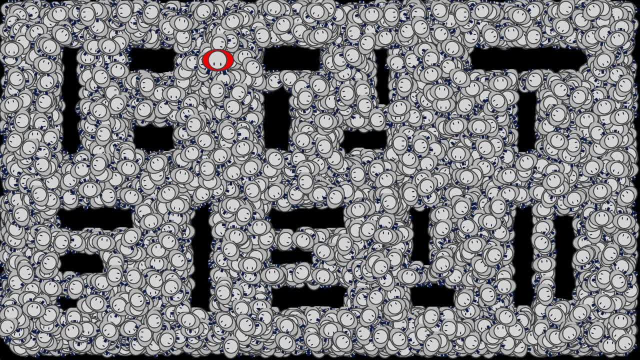 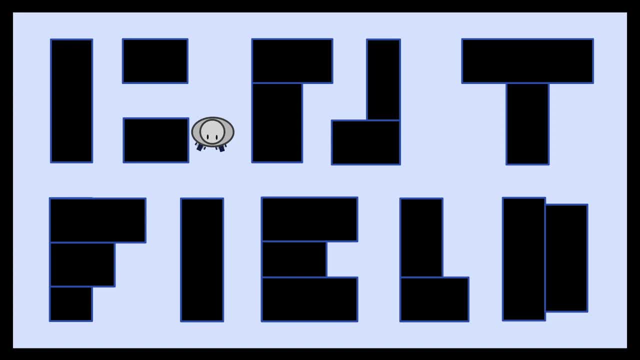 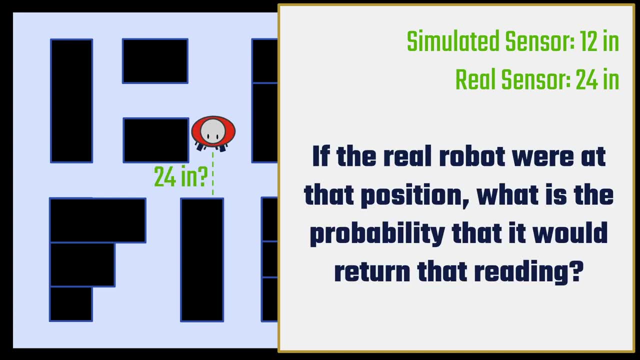 help you find which simulated robot is closest to the real robot's position. This step is called redistribution. I'll show you an example. Here's a simulated robot whose sensor reads 12 inches. This sensor on the real robot reads 24 inches. You have to find out if the real robot were. 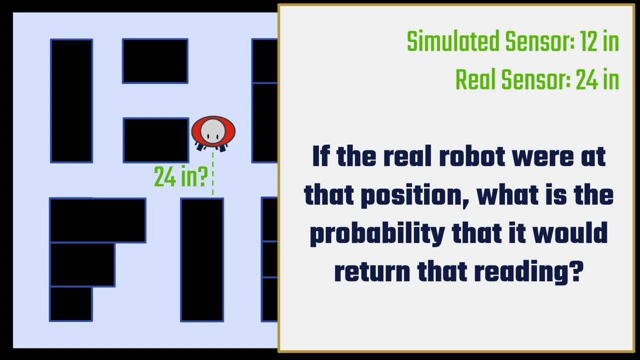 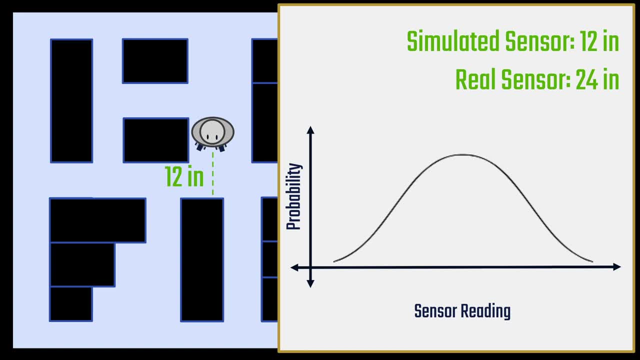 at the simulated robot's position, what is the probability that it would return the real sensor's reading? This probability can be found using the bell curve. Just set the center of the curve at the simulated sensor's reading, or 12 inches, and then, depending on the amount, 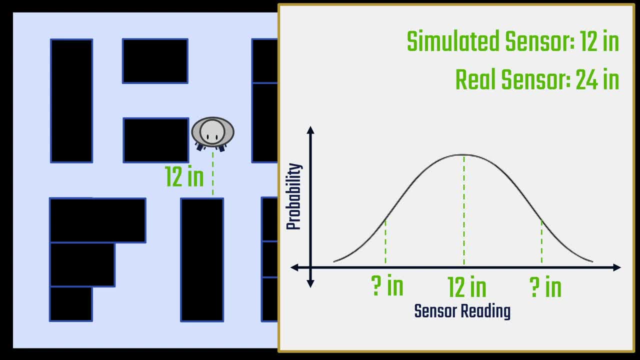 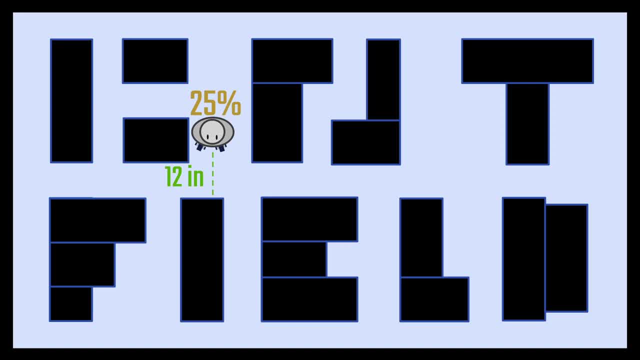 were at the same location as the simulated robot, it would have a 25% chance of getting a reading of about 24 inches. If we add a few other robots here, they have different percentages based on their readings. Now remember these percentages describe how similar the real sensor readings and the 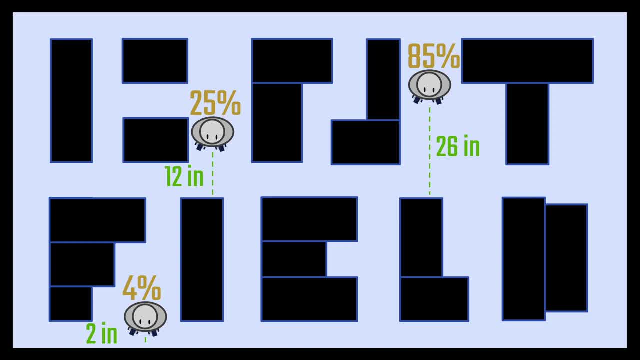 simulated sensor readings are to each other and not where the robot is. The robot could be near or very far away from the robot, but the robots on the real robot are very close to each other. I'm going to hit continue and onto sample estimation by overclocking my 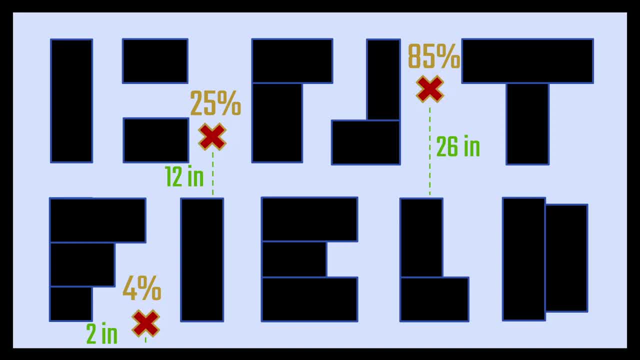 we robots. The robots are removed from the map and then placed back on the map according to the probabilities. Positions with higher probabilities are more likely to have one or multiple robots placed there, and the robots will be placed in exactly the same location. I've overlapped them a little bit here, so you 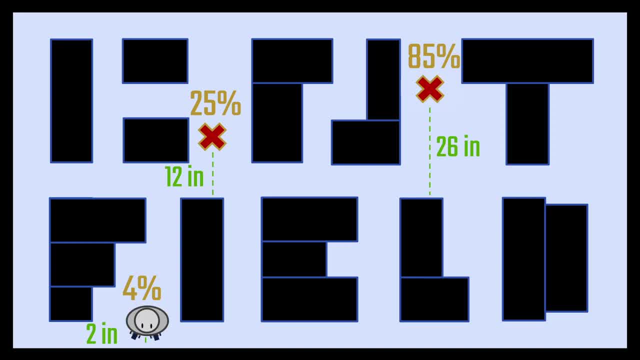 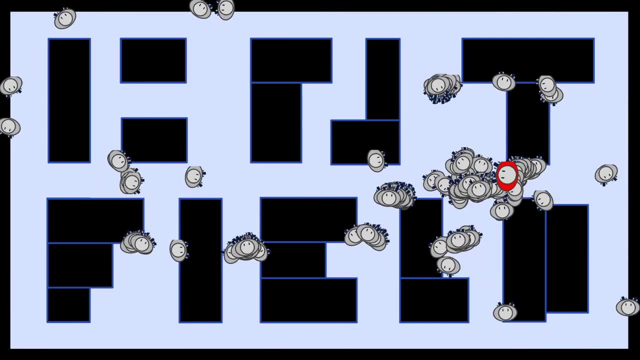 can see that there are multiple robots. Positions with low probabilities are unlikely to have a robot. so maybe this is the final distribution of robots. Then the robots can be moved, redistributed, moved and redistributed again and again in a loop. Over time the robots begin to cluster around a single spot. Sometimes 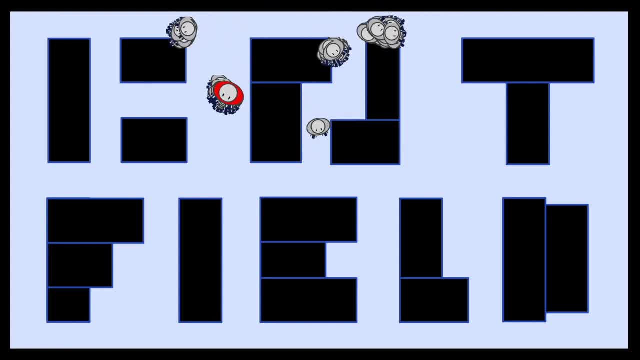 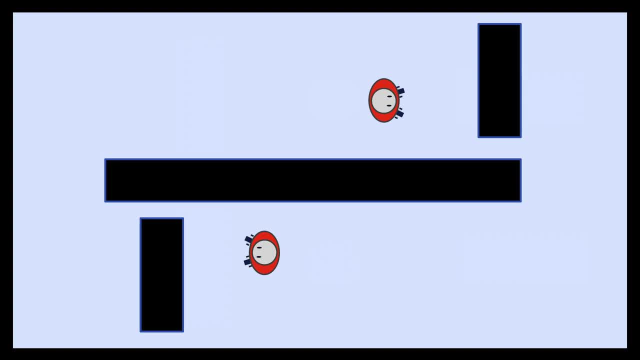 other clusters might break off into areas that look similar to the one the real robot is in, but they disappear as the robot moves into a new area. The exception to this is when the robot is driving somewhere where the map looks exactly the same from several locations. The robot could be in any of these four. 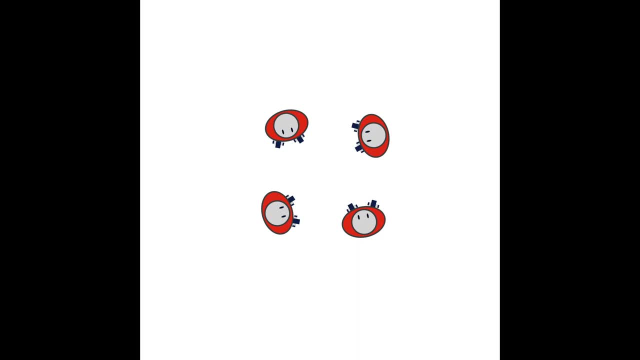 places and the sensor readings would always be exact the same, no matter how the robot moves, If there ends up being only one cluster. where the final cluster ends up is actually just a matter of chance, If the clusters don't form in the right, 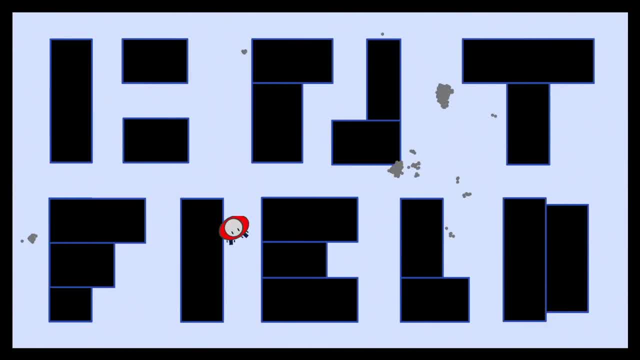 place. you can increase the number of robots, or you can also make the robots scatter a little bit every time you redistribute the robots. You can also kidnap the robot- that's actually what it's called in robotics- then detect when the cluster is in the wrong spot and re-scatter the robots. 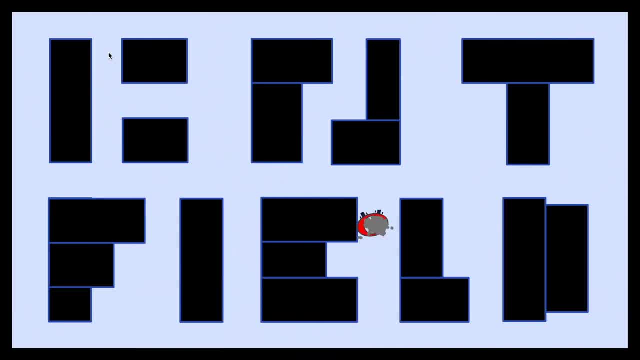 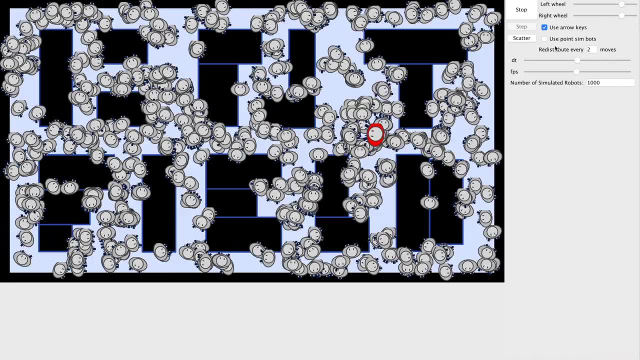 If you're interested in exploring particle filters more, we have the app available for download on GitHub and it's linked below in the description. You can move the robot, control all the simulated robots to look and how they move, and a bunch of other things.